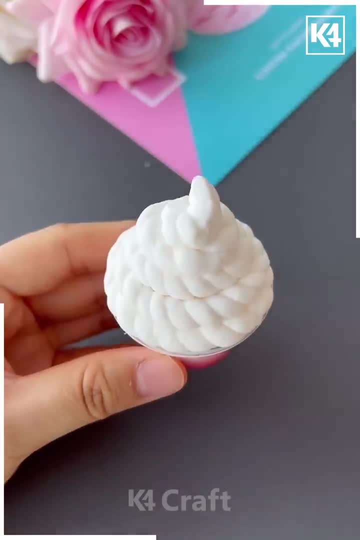 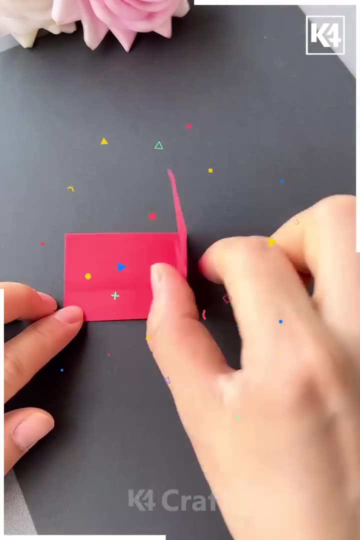 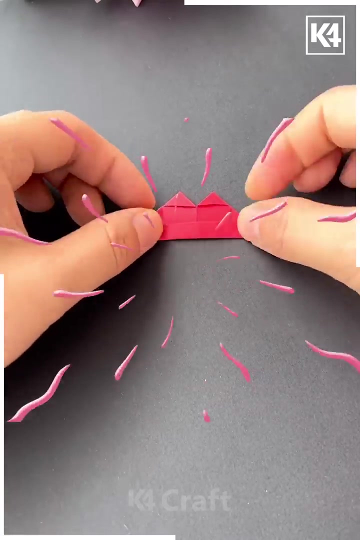 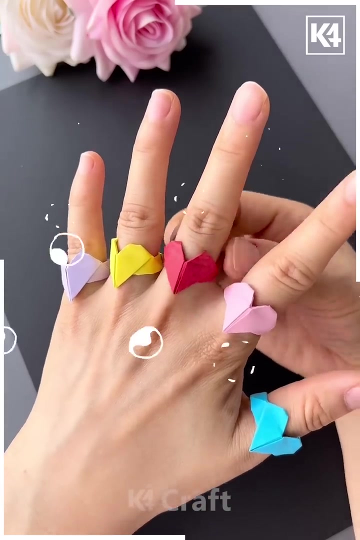 clay and we will paste it on the bowl and you can see the tasty cupcake is ready. Next we will use red colored paper and we will give some folds to it and next we will make a triangular from it and after this we will open it and you can see a beautiful ring is almost ready, and now this is ready. 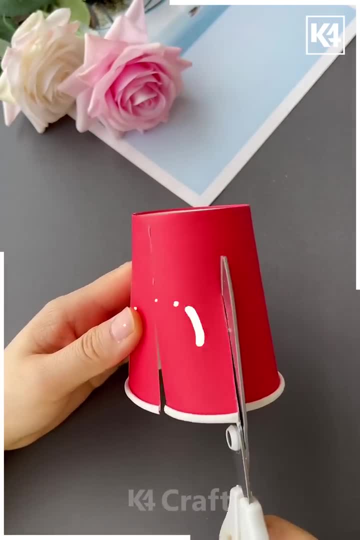 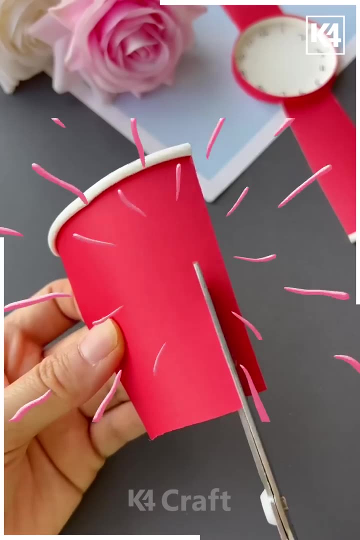 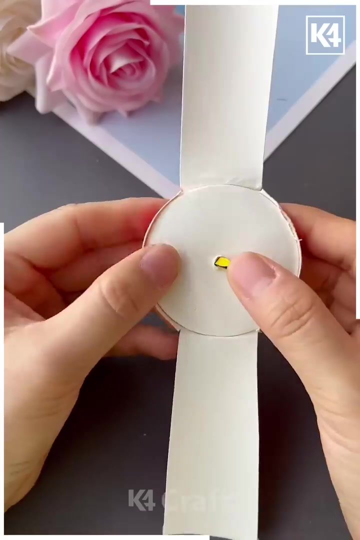 to use. Now, again, we are using a paper cup and we are cutting it from both the ends, and now we will write in the between the time. and this is the watch which is ready to use. You can give this to anyone. This is completed after some textures. 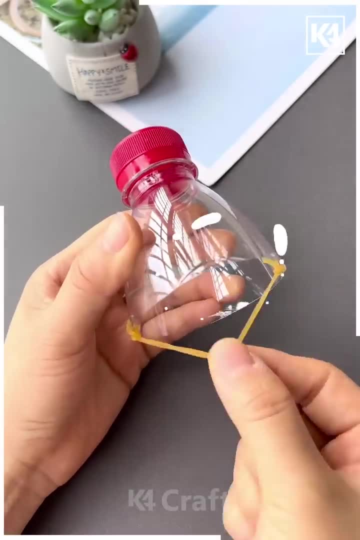 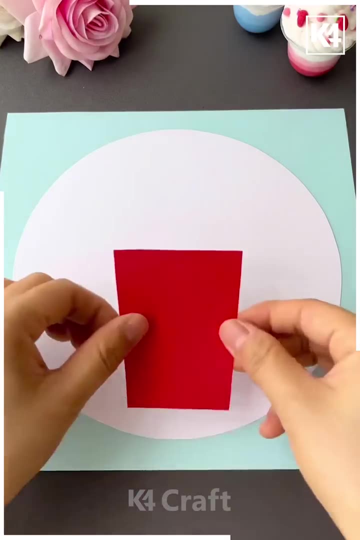 Now we are using a bottle and we are cutting it from the upper part and we will use some paper and we will play it like a bow and arrow. So now again, we are pasting some paper on the base and we are making some watermelon. 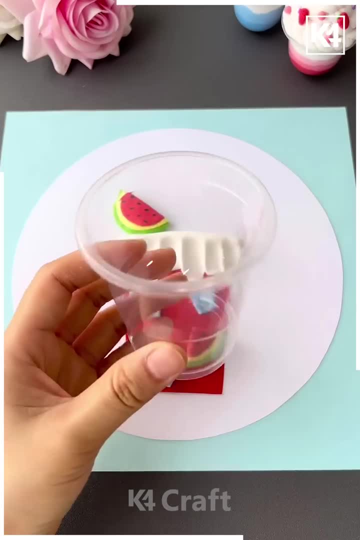 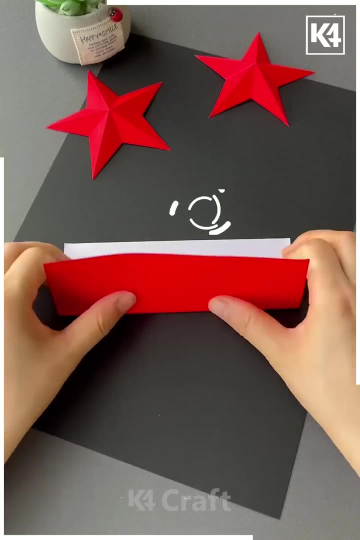 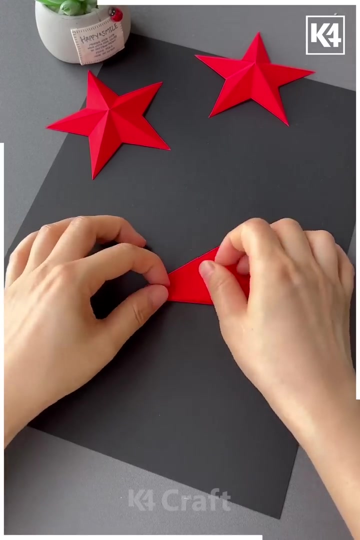 with it, With the clay, and we will paste it all over and this craft is ready now and you can see how delicious this is looking. Next, we will use a red color paper to make the star, The similar star which is kept on the table. 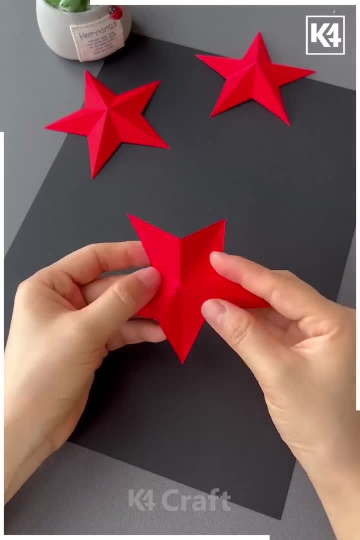 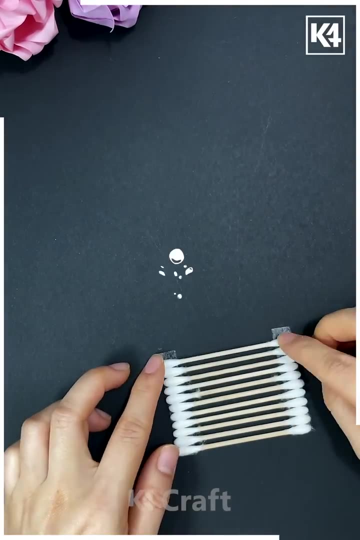 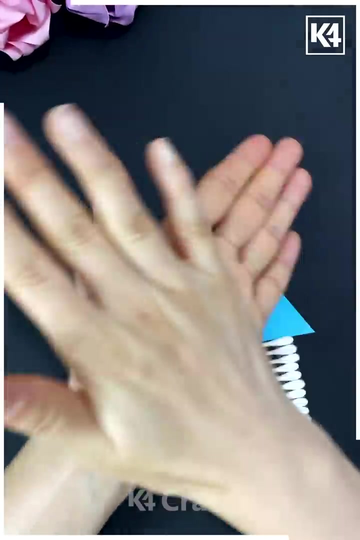 It is very easy to make. You can see, we have cut it and we have already made the star. Now we are using some ear bird and we are pasting it On the paper and we are making a house with it. Next we will draw some lines and we will make the balloons with the clay. 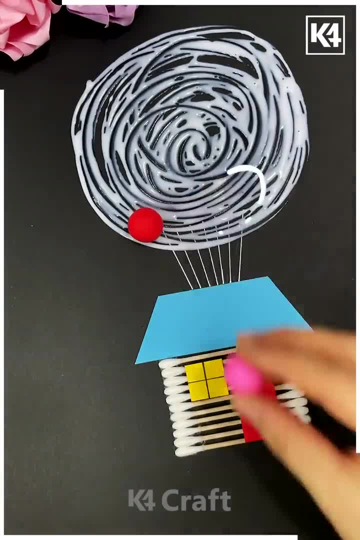 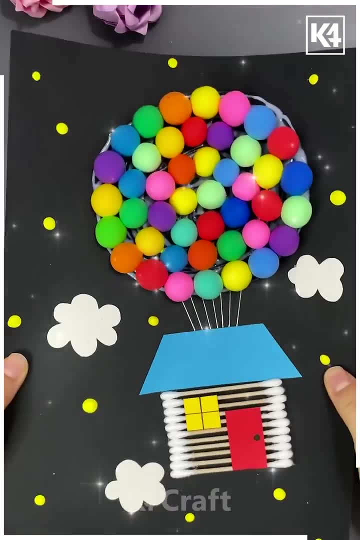 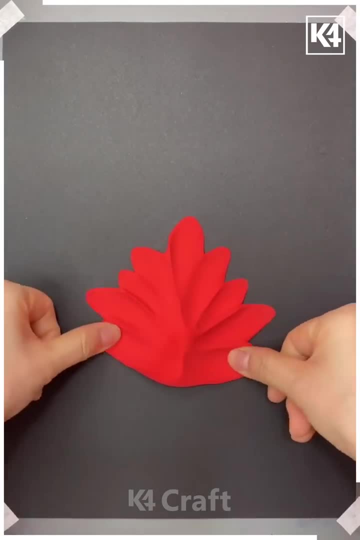 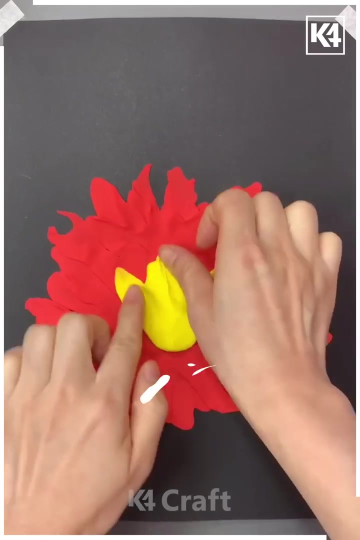 We will paste different color balloons. You can see how good it will look now and this craft is completed. Next, we will use some red color clay and we will paste it on a black color paper and we will spread it with our fingers. We will use a yellow color clay and we will paste it, and we will follow the same steps. 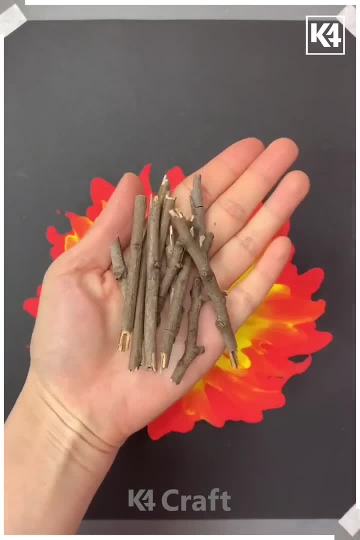 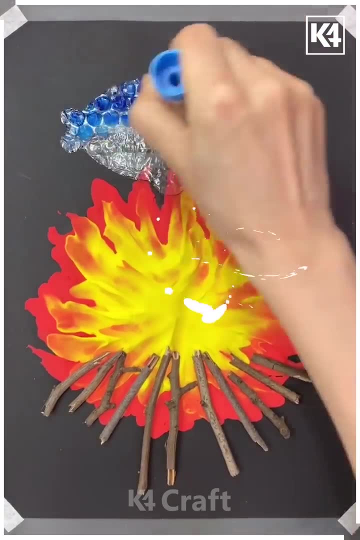 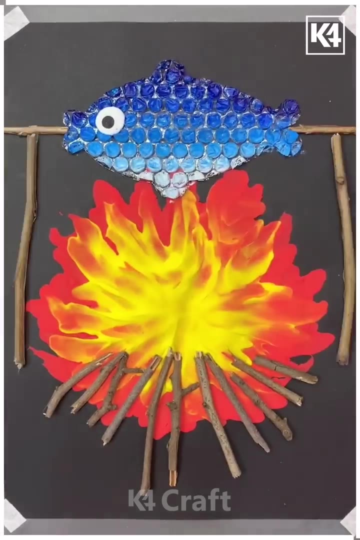 as last one, and next we will paste some wooden sticks to make it look more real. Next we will make a fish from a plastic and we will color it, and then we will add the eyes and some wood and you can see how realistic it is looking now.